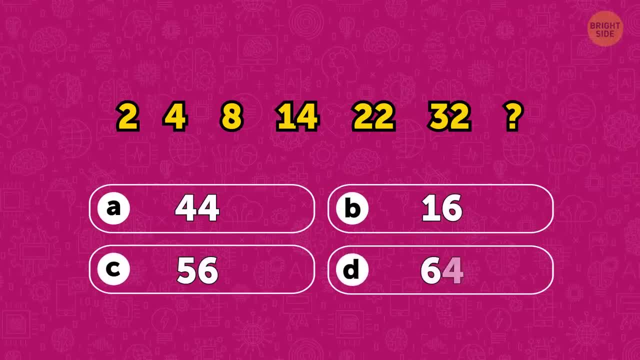 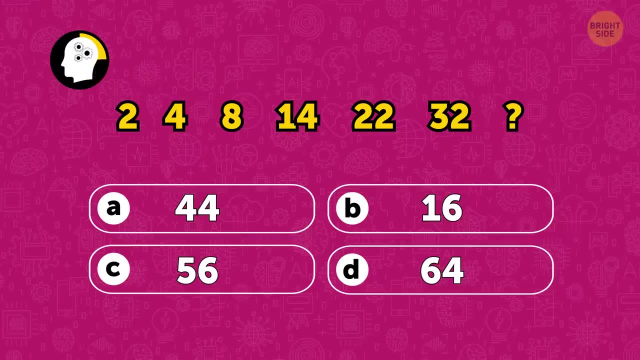 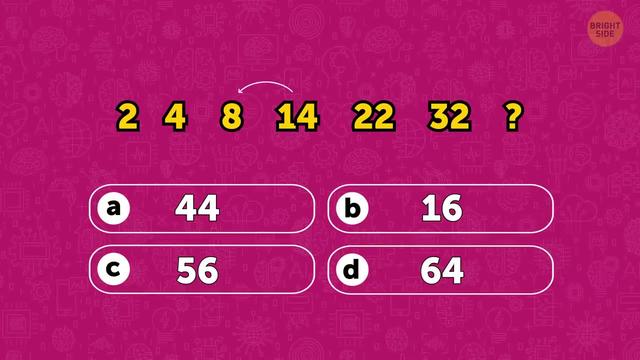 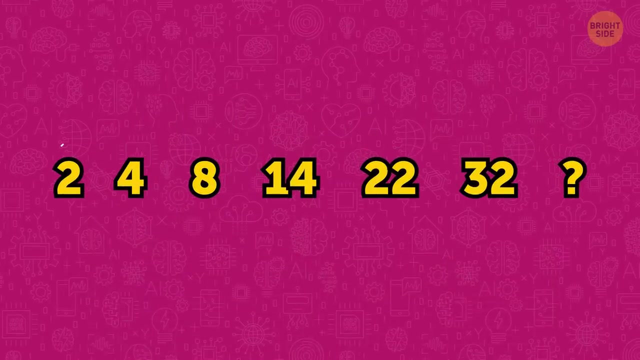 C, 56, D, 64. In this sequence, each number is greater than the previous one. It means that the number you're looking for also needs to be greater than 32.. So the sequence goes like this, And the correct answer is 44.. 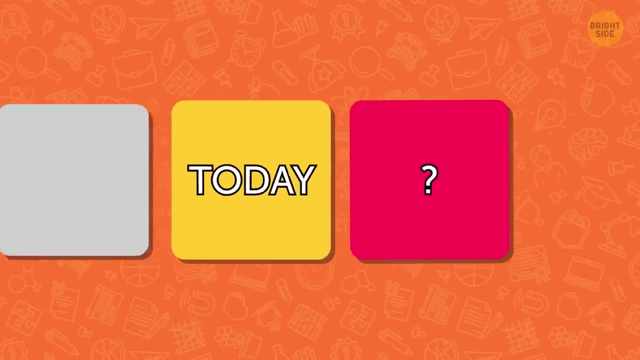 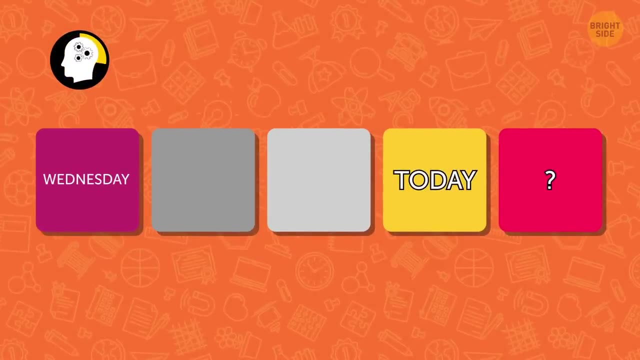 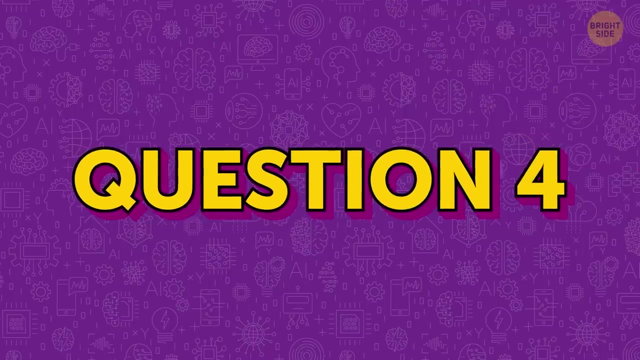 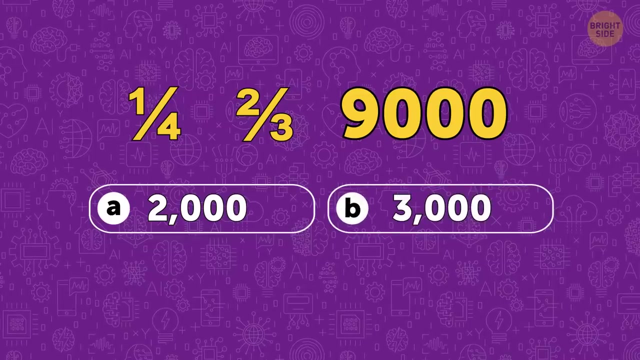 Question 3.. What day will it be tomorrow if Wednesday was 3 days ago? The correct answer is Sunday. Question 4. What is a quarter of two-thirds of 9,000?? A, 2,000, B, 3,000. 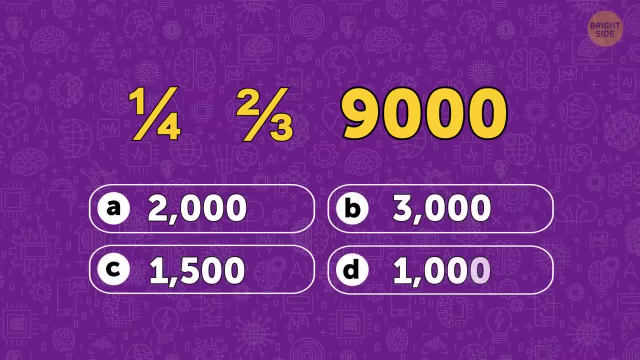 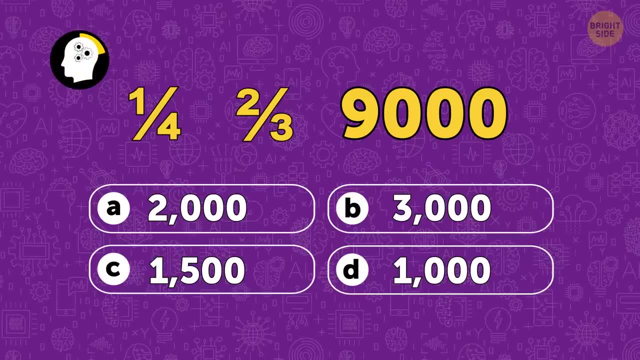 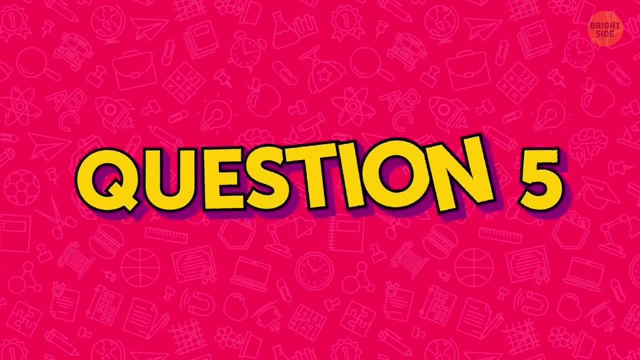 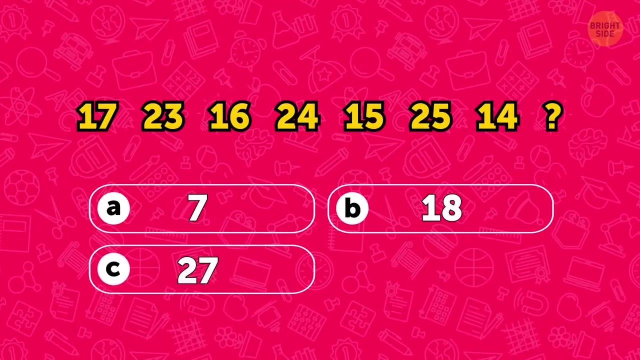 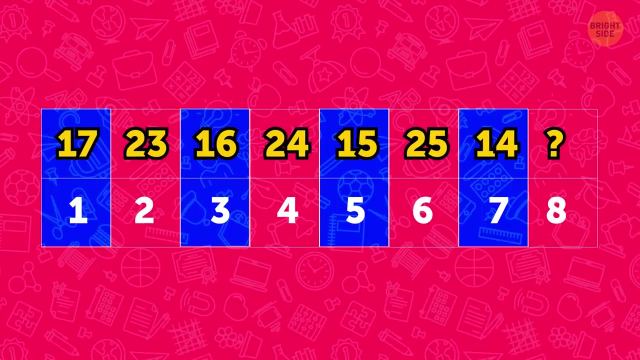 C, 1,500, D 1,000. The correct answer is C, Question 5.. What number should come next in this sequence? A, 7, B, 18, C, 27, D, 26? Take a look at the 1st, 3rd, 5th and 7th numbers first. They decreased by 1.. 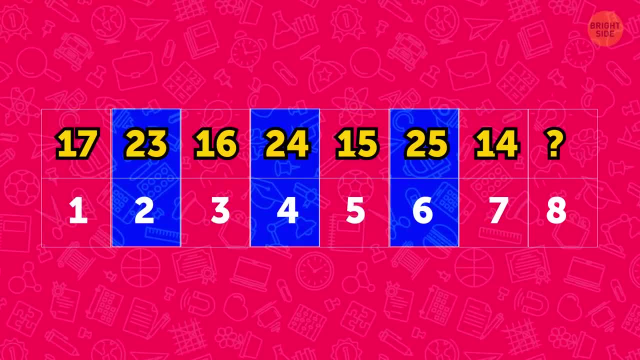 On the other hand, the correct answer is C. On the other hand, the 2nd, 4th and 6th numbers increased by 1.. The number you're looking for belongs to the 2nd group, since it's going to be the 8th number. 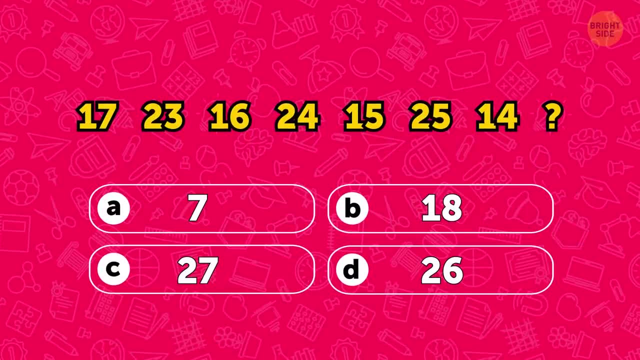 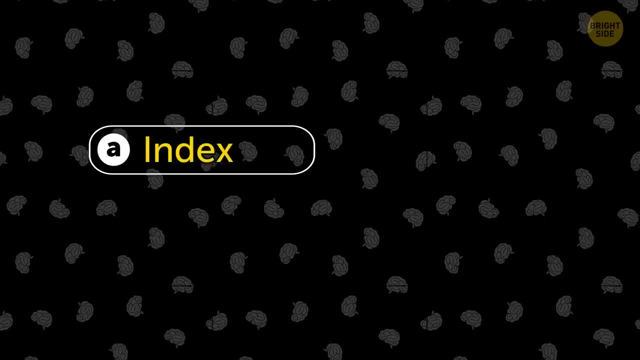 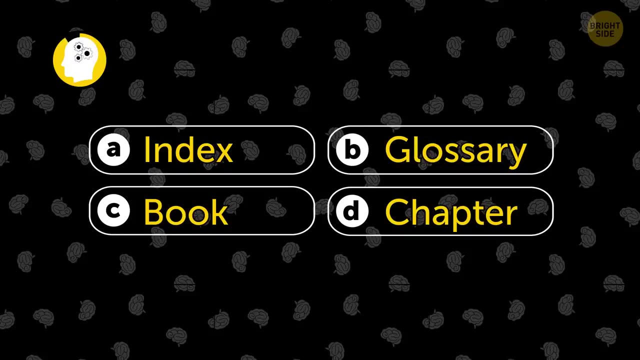 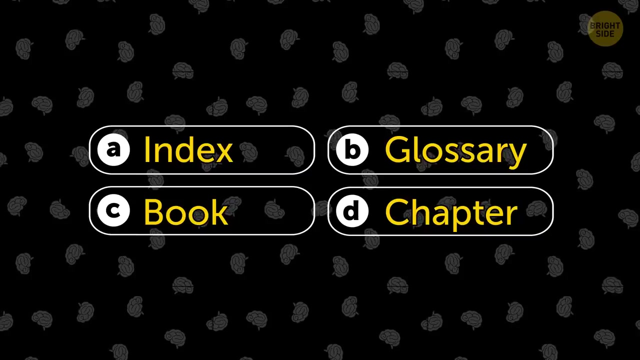 And what comes after 25? 26.. So the correct answer is D, Question 6.. Which word is the odd one? A, Index, B, Glossary, C, Book, D, Chapter? The word book is the different one because the rest of the words are all part of a book. 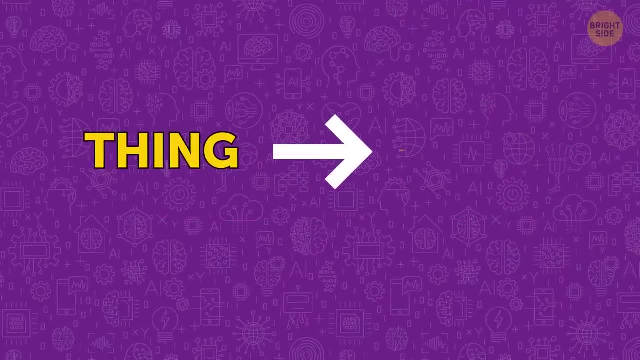 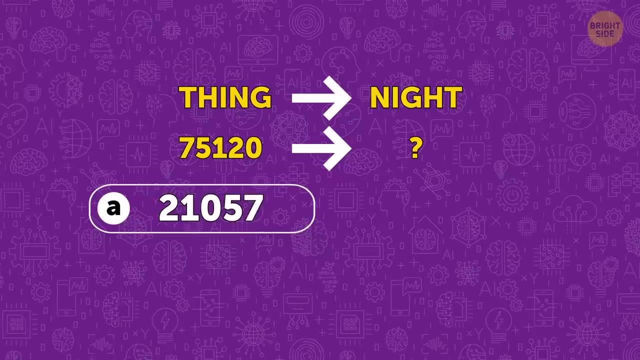 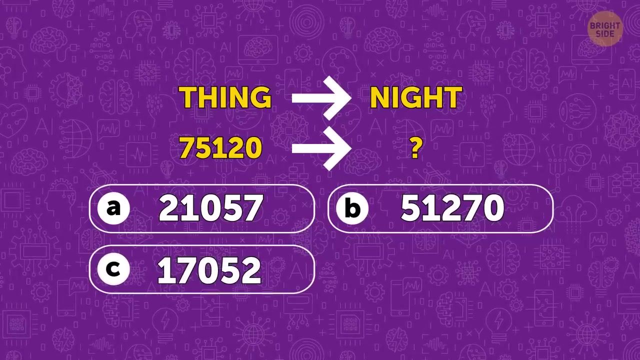 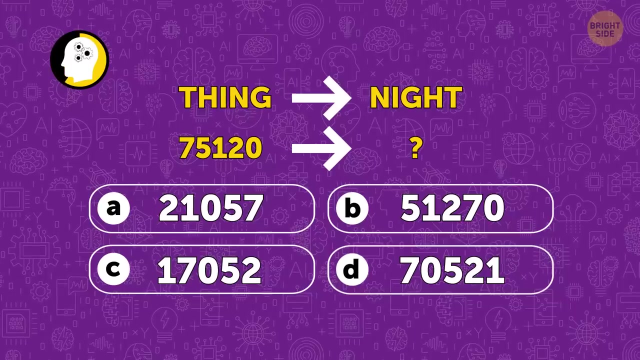 Question 7. If thing turns into night, what does 75120 turn into? A, 21057, B, 51270, C, 17052, D, 705217? Question 8. What is the relationship between the word thing and the number 75120?? 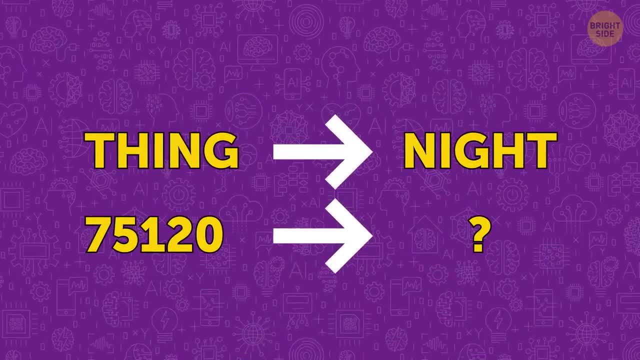 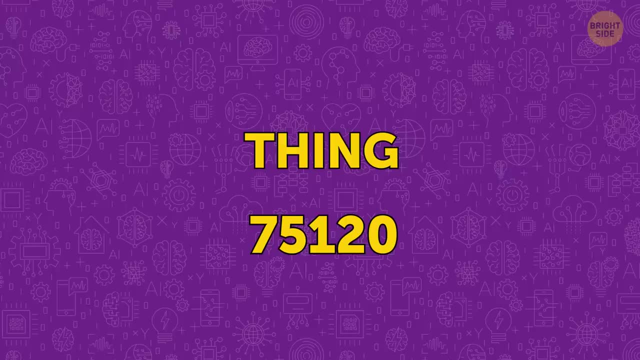 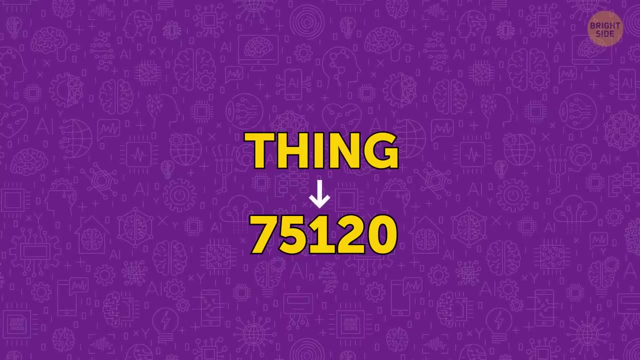 To solve this riddle you need to figure out the relationship between the word thing and the number 75120.. Once you do that, you'll realize that a particular letter corresponds to a certain number. So T is connected with 7, H with 5, I with 1, N with 2, and G. 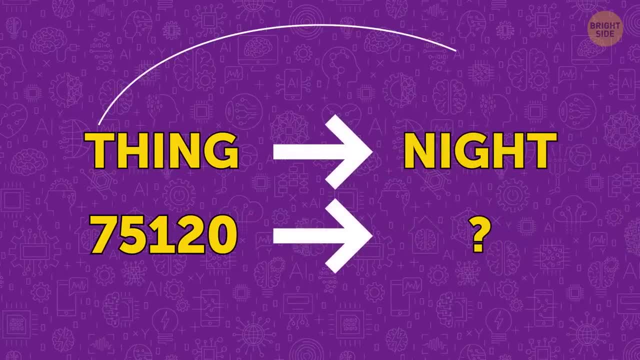 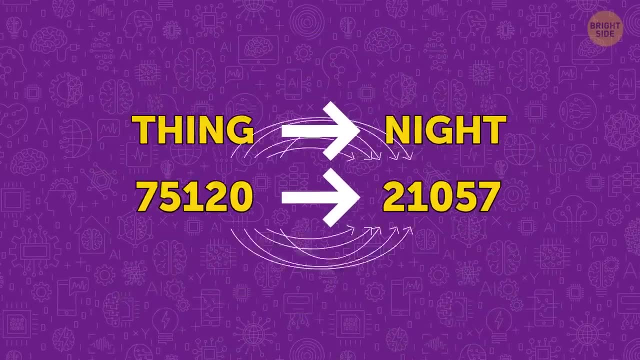 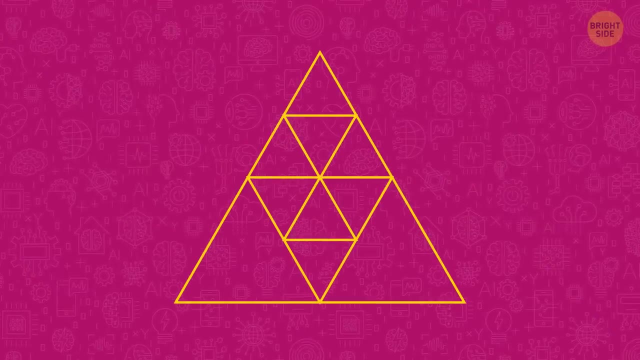 With 0.. Now arrange these numbers according to the order of the letters in the word night. You'll get 21057.. So the correct answer is A Question 8.. How many triangles are there in this picture? A 10. 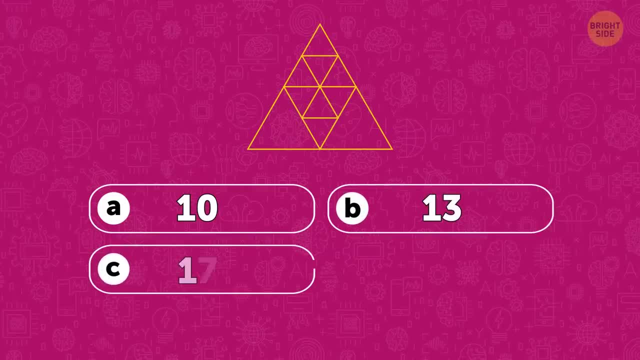 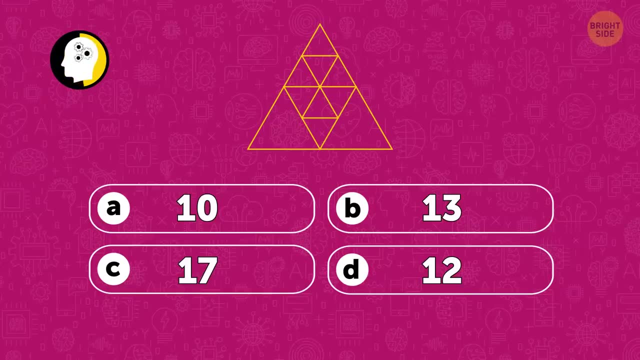 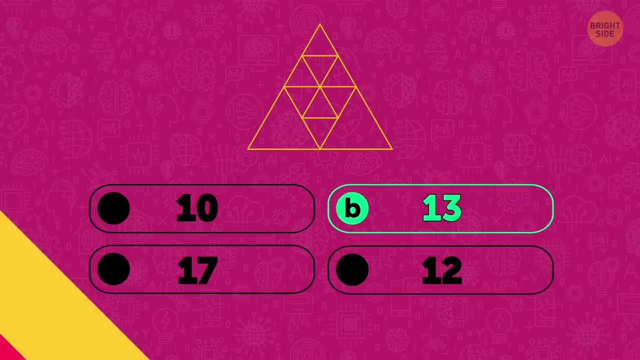 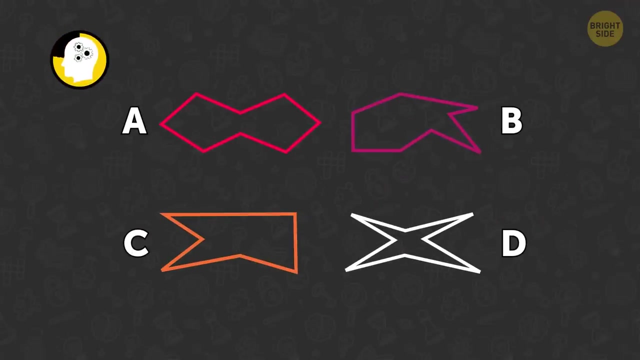 B, 13, C, 17, D, 12. The correct answer is 13.. Question 9. Which shape is different from the others? The correct answer is C, because all the other shapes have 8 sides, while this one only has 6.. 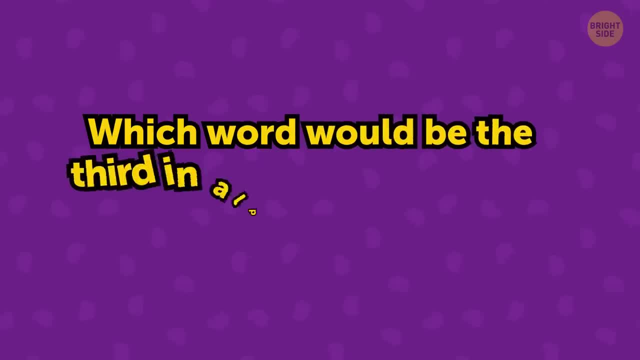 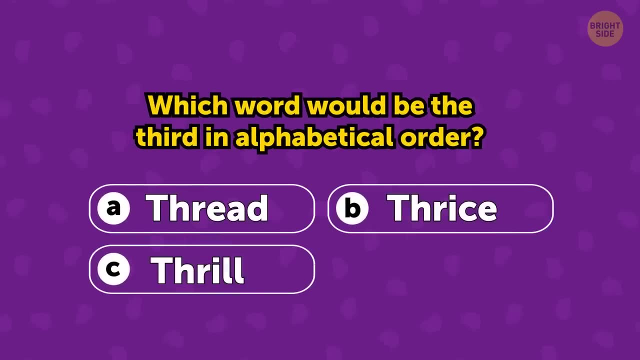 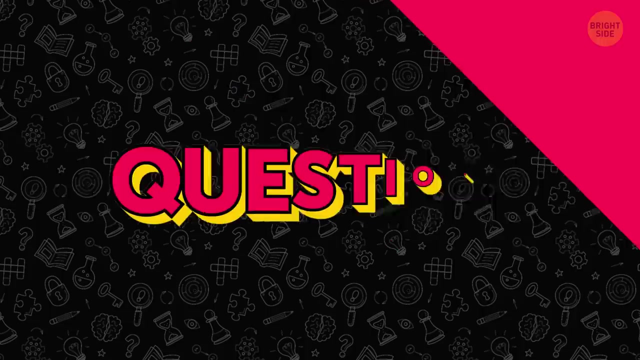 Question 10.. Which word would be the third If you put them in alphabetical order: A Thread, B, Thrice, C, Thrill, D, Thrive? The correct answer is C, Question 11.. A dress and a belt cost $830 in total. 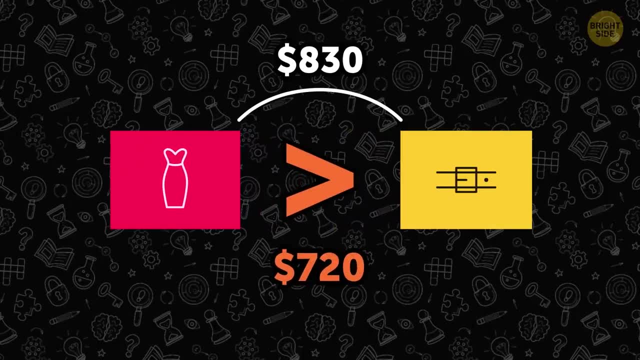 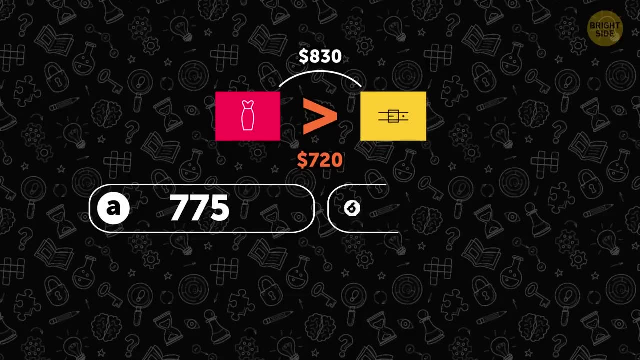 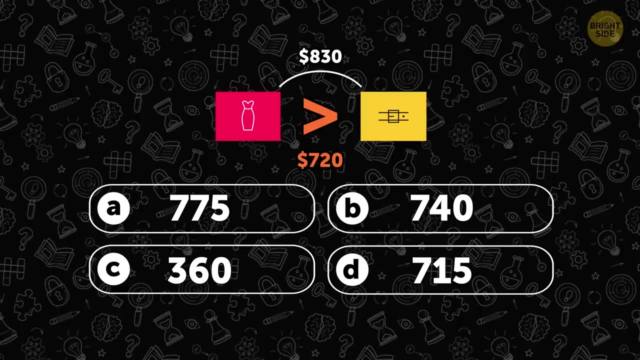 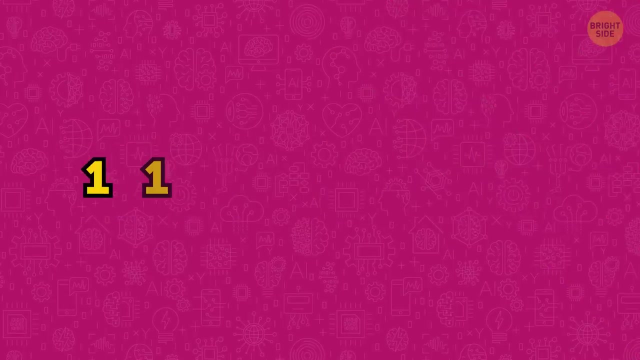 The dress is $720 more. The belt is more expensive than the belt. How much does the dress cost? A, $775, B, $740, C, $360, D, $715. The correct answer is A Question 12.. What number is the next in this sequence? 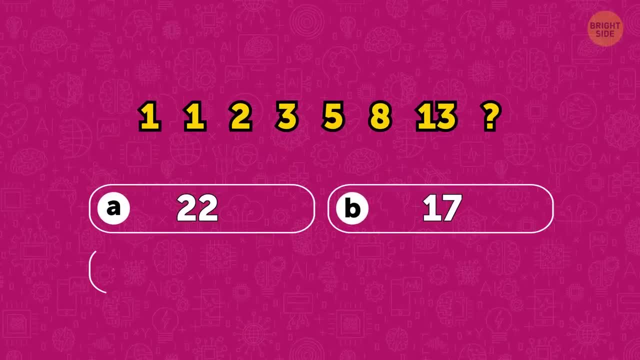 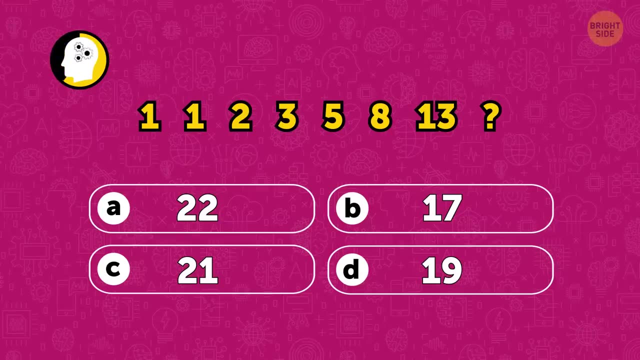 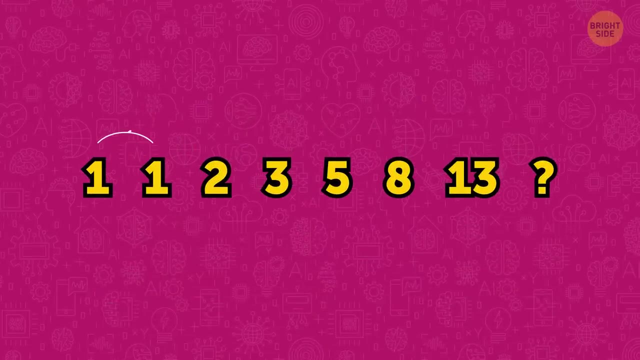 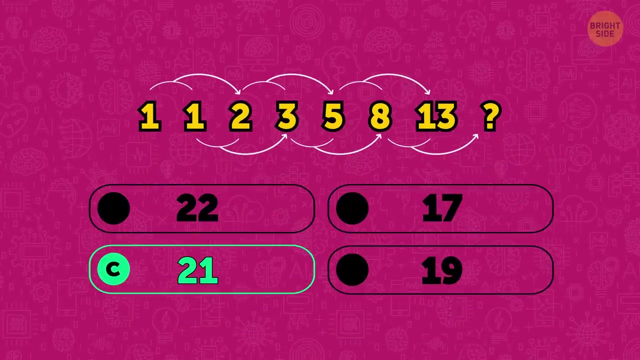 A, 22, B, 17, C, 21, D, 19. Each number is the sum of the two numbers that comes before. When you add 8 to 13, you get 21.. So the correct answer is C, Question 13.. What is the number you need? 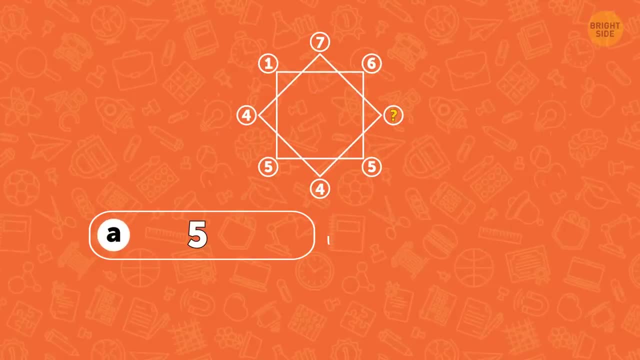 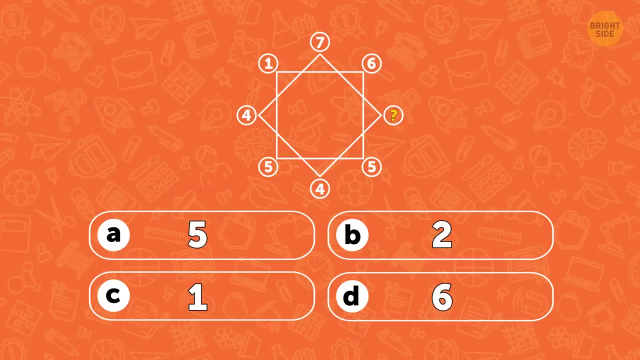 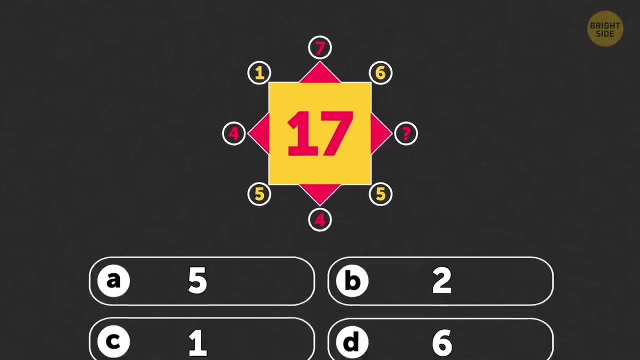 A, 5, B, 2, C, 1, D, 6. Do you see the two squares? The sum of the numbers in their corners needs to equal 17.. So that makes 2 the correct answer. Question 14.. Question 15.. 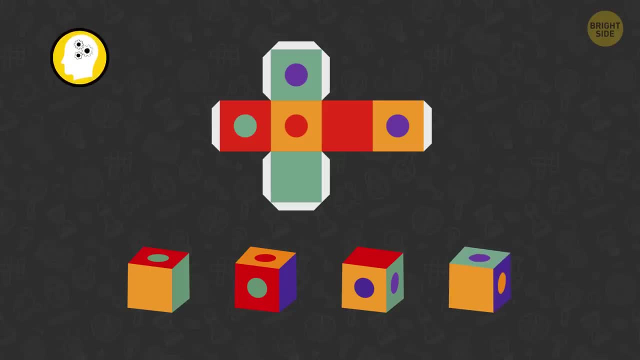 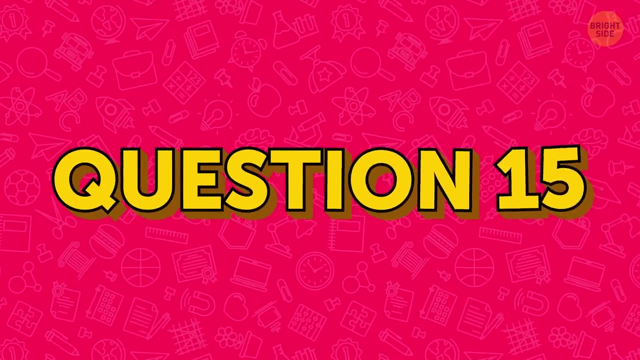 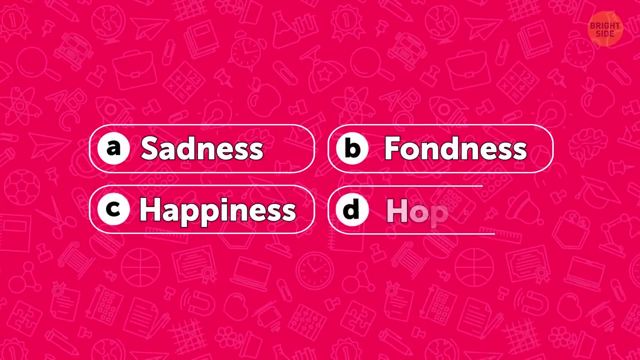 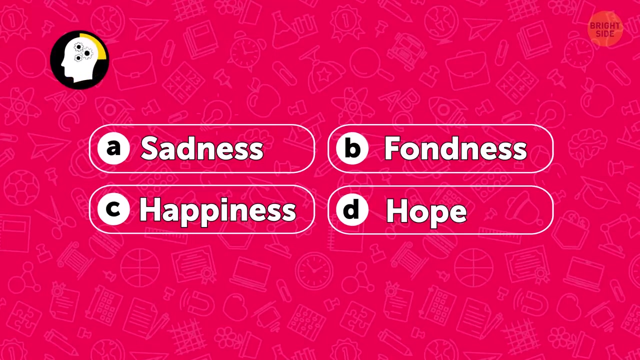 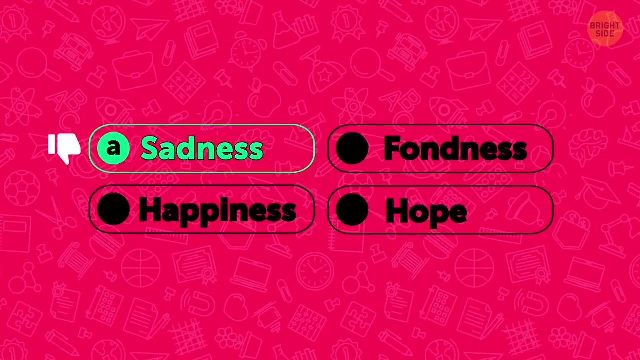 Question 16.. Question 17.. What is the finished cube going to look like? The correct answer is C. Question 15.. Which word is the odd one? A- Sadness, B. Fondness, C- Happiness, D- Hope. The correct answer is Sadness, since it's considered to be a negative emotion, while the rest of them are positive feelings. 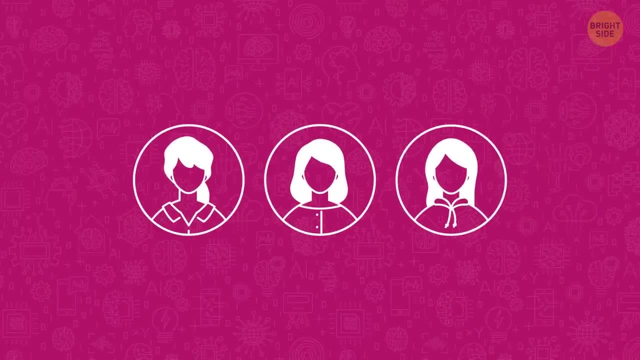 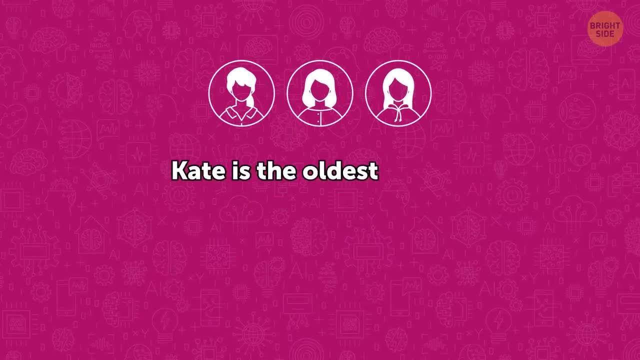 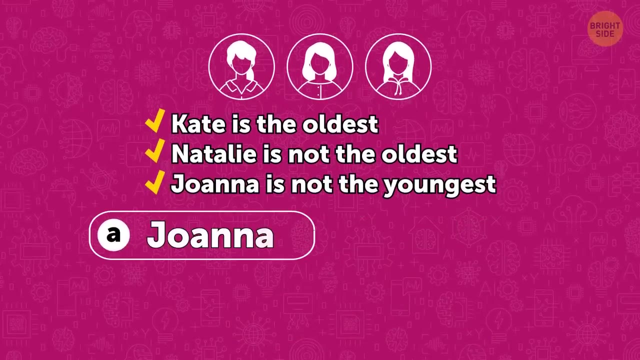 Question 16.. Kate, Joanna and Natalie are three sisters. If the following statements are all true, which of them is the youngest? Kate is the oldest. Natalie is not the oldest. Joanna is not the youngest. A. Joanna B Hannah. 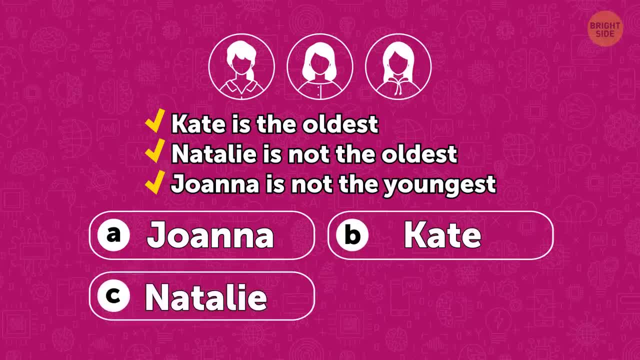 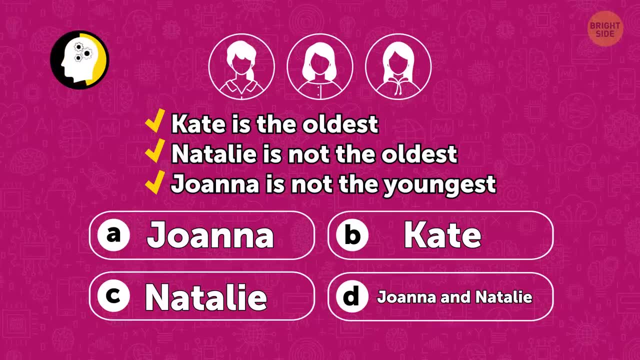 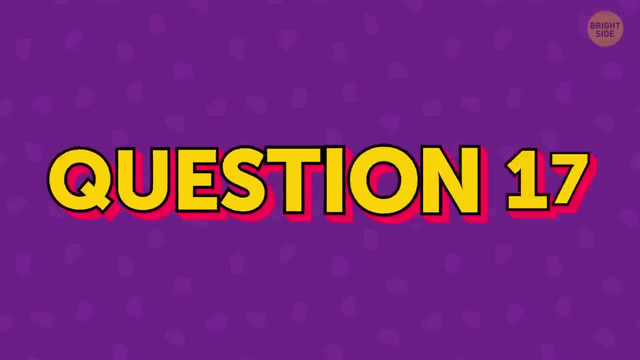 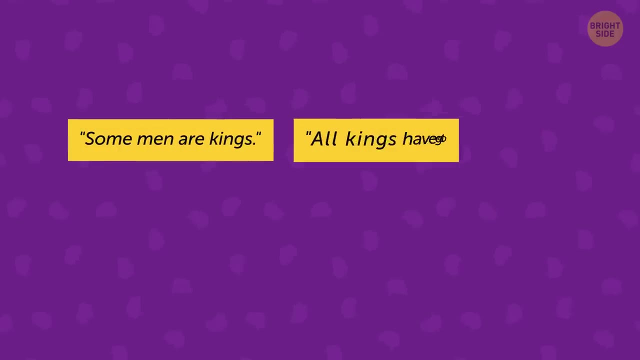 C. Kate C. Natalie D. Both Joanna and Natalie. The answer is Natalie, Question 17.. Here are two statements: Some men are kings, All kings have golden crowns. And here are two conclusions: All men are kings And men have golden crowns. 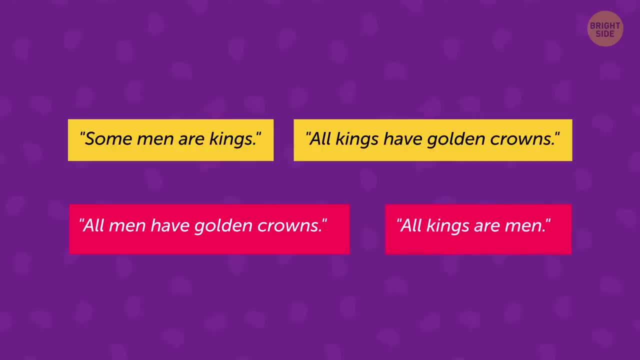 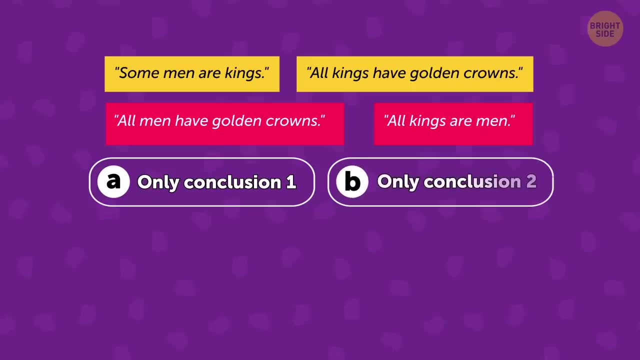 All kings are men. Which of the following is the correct answer? A- Only conclusion. 1. B- Only conclusion 2. C- Either 1 or 2. D- Neither 1 nor 2. E- Both 1 and 2. The correct answer is D. 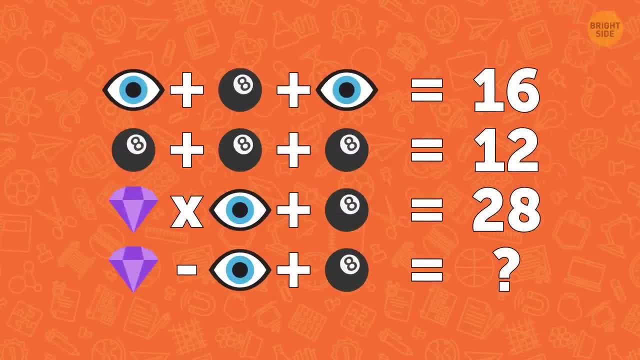 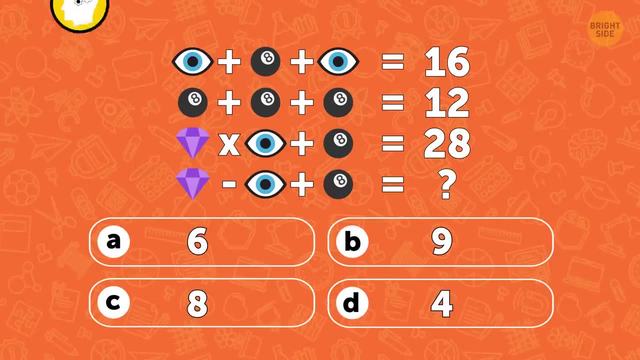 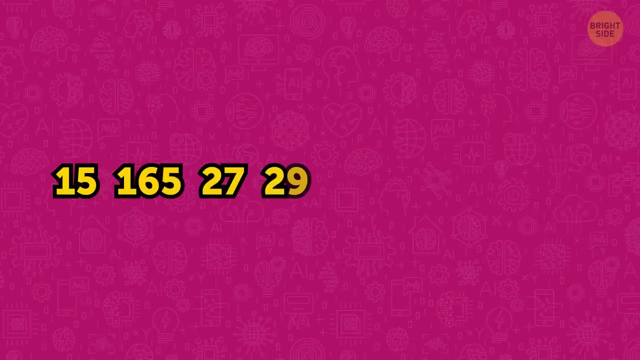 Question 18.. What is the result? A, 6, B, 9 C, 8, D, 4. The correct answer is A Question 19.. What number comes next in the sequence: A, 2, A, 47. 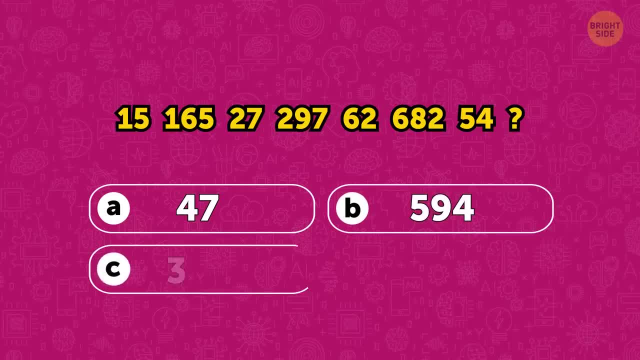 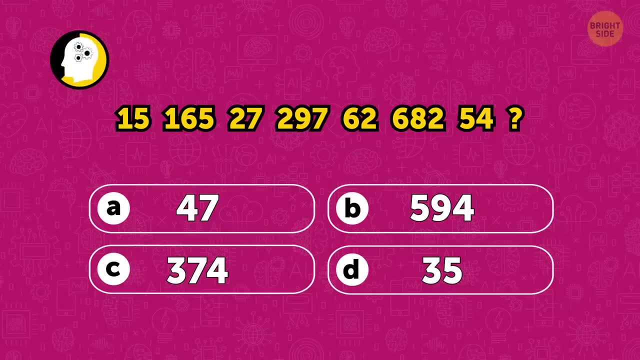 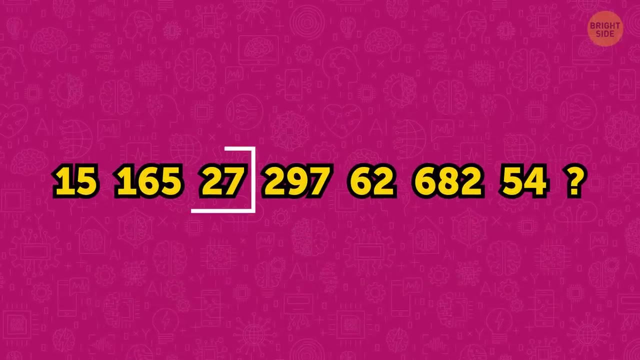 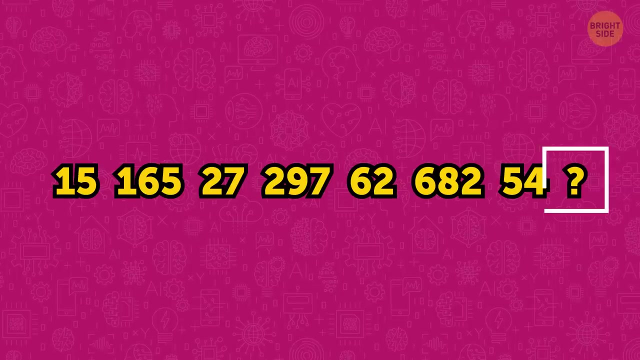 B 594 C, 374, D, 35, Question 20.. What number comes next in the sequence? In this sequence, a two-digit number is followed by a three-digit one, and vice versa. So the number you're looking for has to consist of three digits, as the one that comes before is a two-digit number. 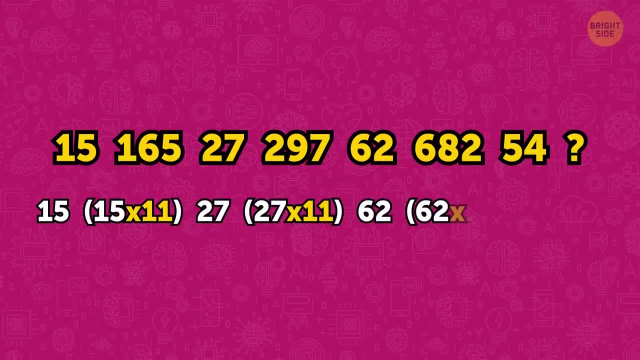 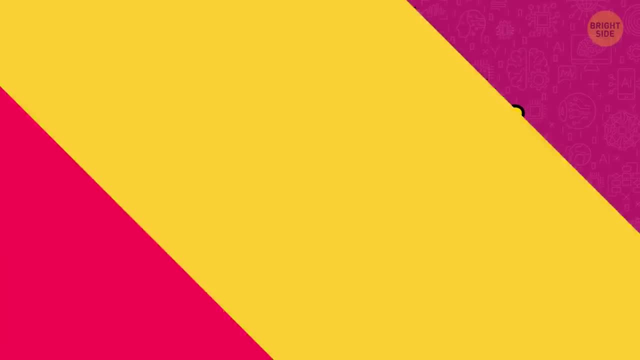 And the formula for this sequence of numbers is. The formula for this sequence of numbers looks like this. So what you have to do is multiply 54 by 11.. That makes B the correct answer. Question 20. Identify the shape that continues the sequence. 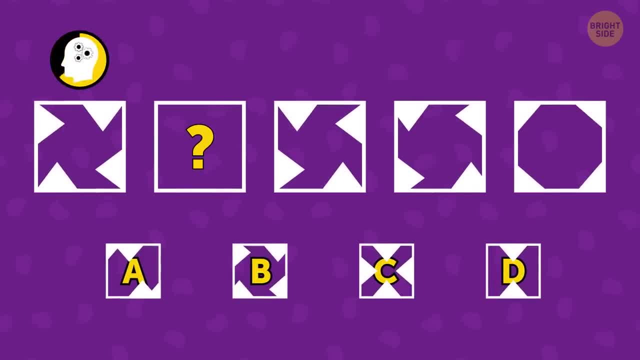 Question 20.. Identify the shape that continues the sequence. The correct answer is B. Congratulations, You've completed the test. Hope you remember your score. Here are the results: Congratulations, You've completed the test. Hope you remember your score.